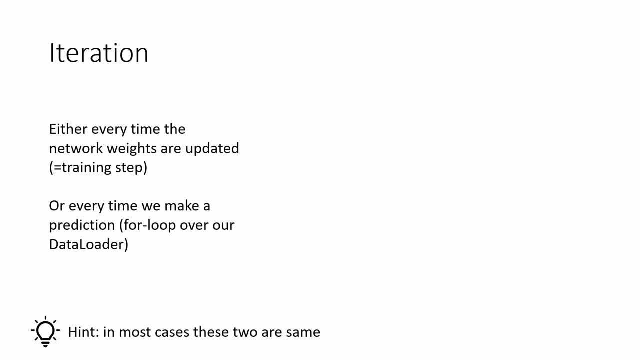 you have seen the whole data set before making an update, in which case these two definitions would be different. We have multiple for loops over the data loader, but then at the end, only one update of the network weights. If you are a beginner, just think of an iteration as one loop. 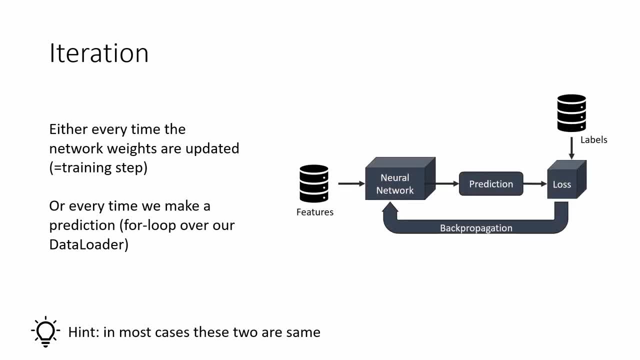 through this training cycle on the right. Also, most research literature I've read often talks about training cycles. If you are a beginner, just think of an iteration as one loop through this training cycle on the right. Also, most research literature I've read often talks about training. 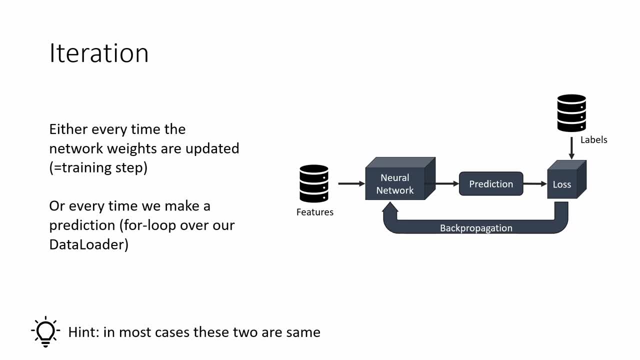 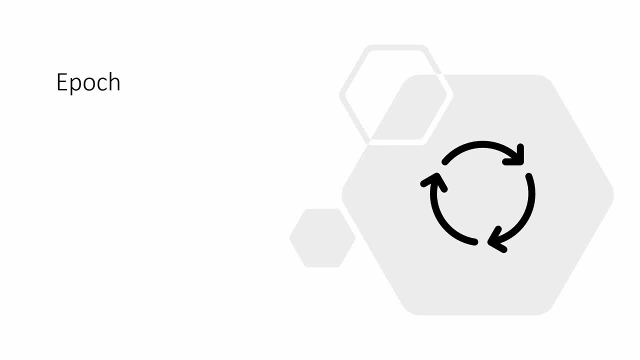 steps to specifically mean the times when we update the neural network weights. so I would encourage you to use that term as well. Next is the epoch. An epoch is finished once the neural network has seen all the data once. Typically, we are not finished after that because gradient descent. 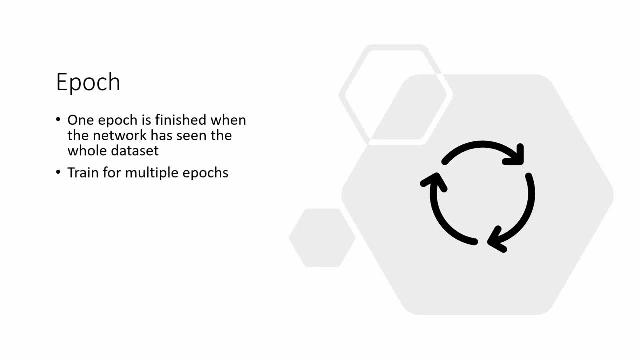 variants only take small update steps and we usually need more updates than are possible within one epoch to reach a good model. So we train for multiple epochs and it's hard to give a number because it's very dependent on the network size and training data. However, it's often more than. 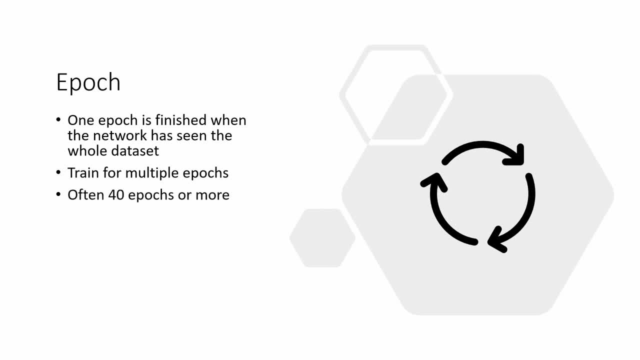 40 epochs. I personally have trained some small image classification models on my local hardware and I used between 5 and 40 epochs, just to throw this out as a super rough estimate. It's also very different how long an epoch takes in terms of time. It could be just seconds or even 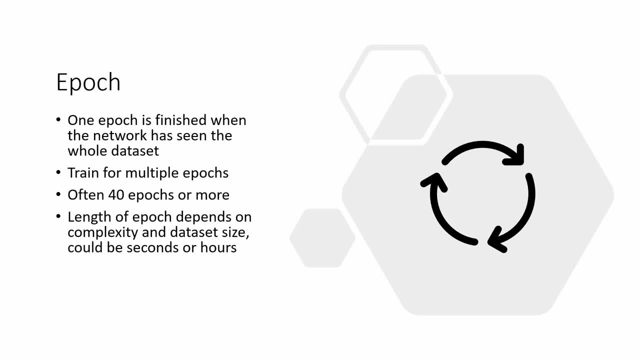 hours per epoch. again, That's very dependent on the type of network being trained and the data set. Overall epochs are a nice metric to describe training length, so they are often used in papers and such because they are independent from the batch size and the concrete layout of iterations. 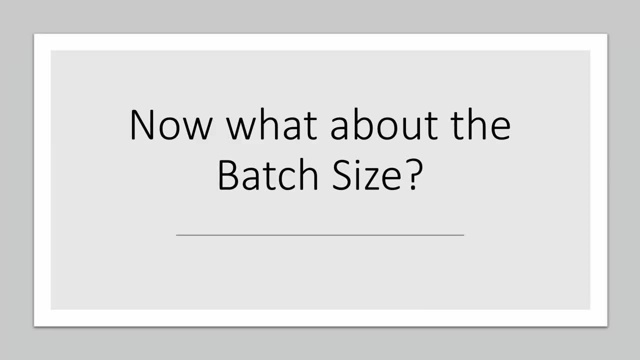 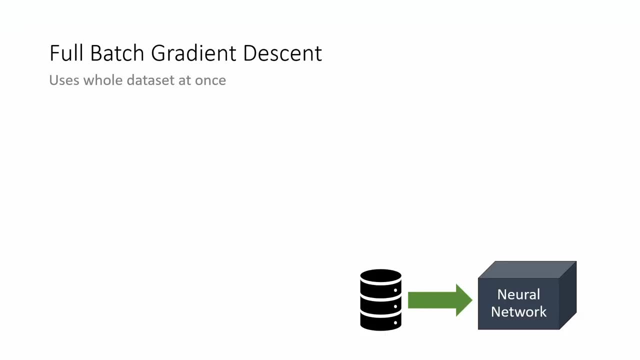 We have talked about iterations and epochs, but what about batch size? There's a bit more to talk about here. We need to show the training data to the network, and one of the ways we can do this is with full batch gradient descent. For that we use the full data set at once. 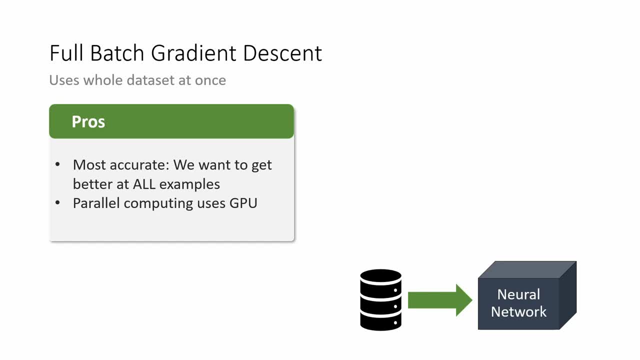 The pros are that it is the most accurate at minimizing the training loss function. After all, we want the network to become better at all the training examples and not only some of them, So it needs to take all of them into account when optimizing. We can also calculate many of the example predictions on parallel with GPUs. 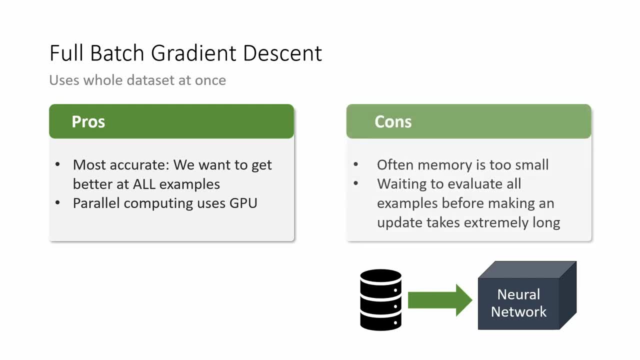 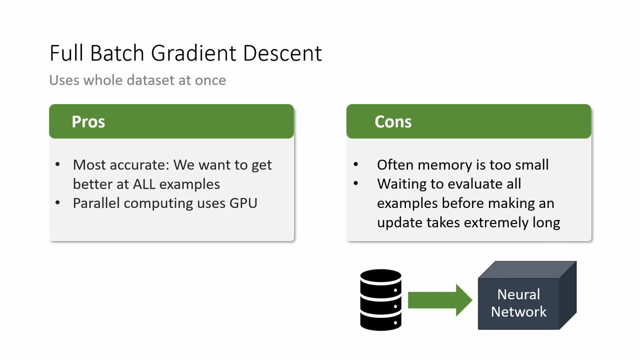 will not fit into memory completely. As I mentioned before, we could also split them into batches and then accumulate the gradients and only do an update at the end. However, that would take extremely long because gradient descent needs to take many training steps to get good, and if every training step takes super long, it's just ineffective. 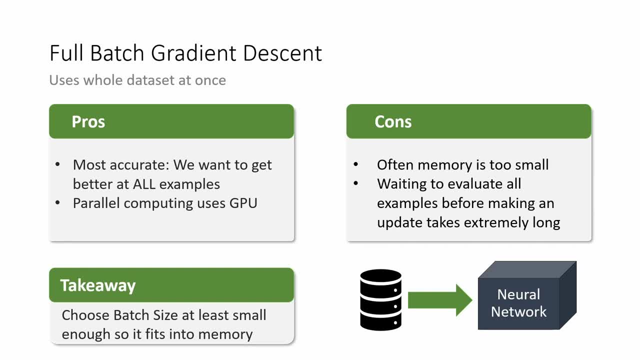 The main takeaway from this is that you need to choose the batch size- at least small enough so you don't run out of memory. Now let's look at what happens if we don't wait with our network update until we have seen the whole data set In Stochastic Gradient Descent. we only 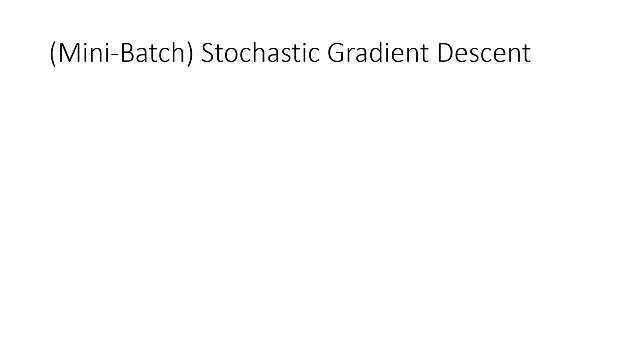 select one data point randomly for each training update. Most of what I say now also applies to the often used mini-batch Stochastic Gradient Descent. In this algorithm we choose a random selection of points from the data set. How many depends on the batch size that we choose for our problem. 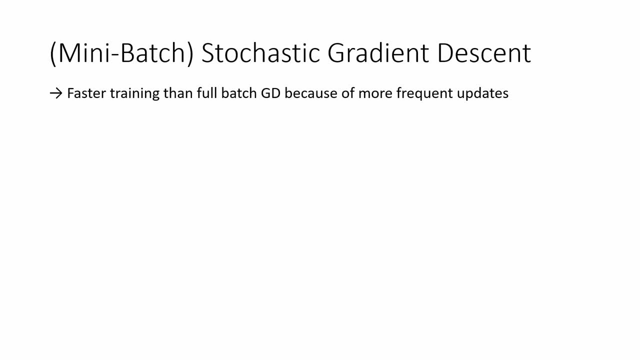 The main advantage originally for this algorithm was that we can train faster by making more frequent updates, even without having complete information about the whole data set. This speeds up training, But what happens to our accuracy? First? it's not as good as gradient descent because, like I said, we make updates before having all the information. 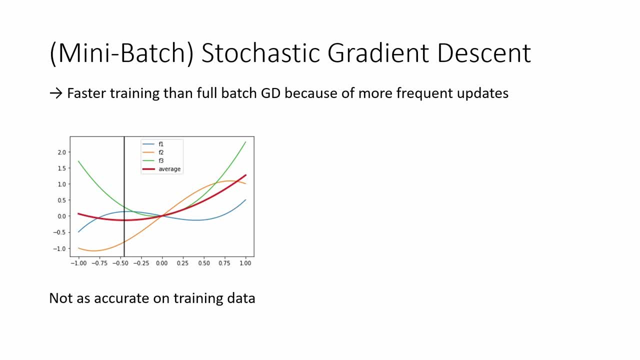 In this plot you can see three different functions- f1, f2 and f3- and they represent a loss of just one data point and you can see the average of those three in red, which would be the loss over all data points that we want to minimize. So, ultimately, we want to minimize the red line to reach the 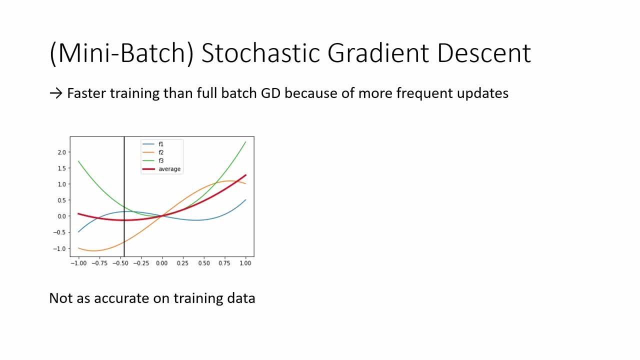 red line at almost x equals negative 0.5.. However, if we look at what would happen if we follow one of the other lines to their minimum, then we can see that they would lead us in different directions, sometimes even in the opposite direction of where we want to go. But since we only take small steps,